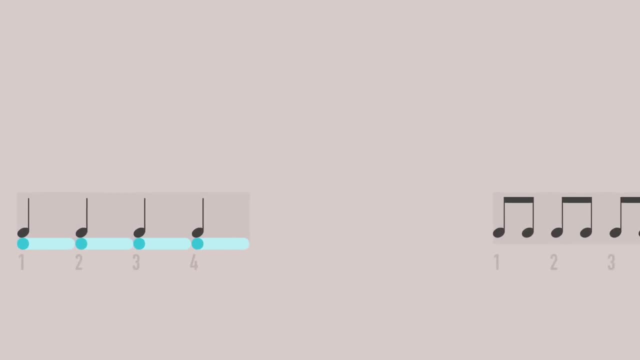 41,, 42,, 43,, 44,, 44,, 45,, 44,, 46,, 47,, 49,, 50,, 51.. We're counting every beat, but when a note lasts for only half a beat, we need a way to. 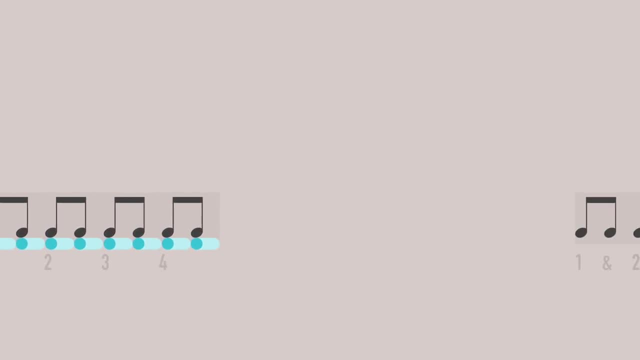 count in between the beats. The simplest way to do this is to count like this: One and two and three and four, and The number lasts for half a beat And the and lasts for half a beat. Let's put all these notes together now. 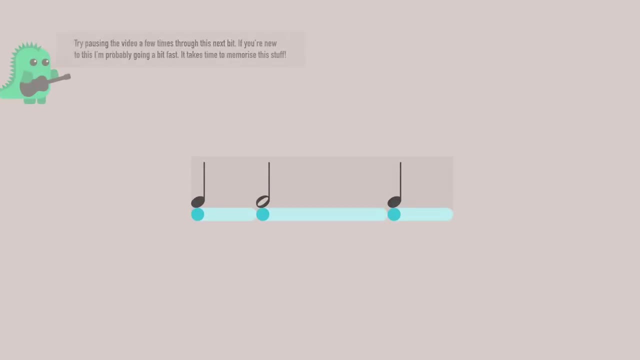 into a short piece of music. Let's look at a short piece of music. Let's go Remember: we have to fill up every bar with notes and the beats have to add up to four. We've only looked at note symbols so far. They make sound, But if we want to stop the 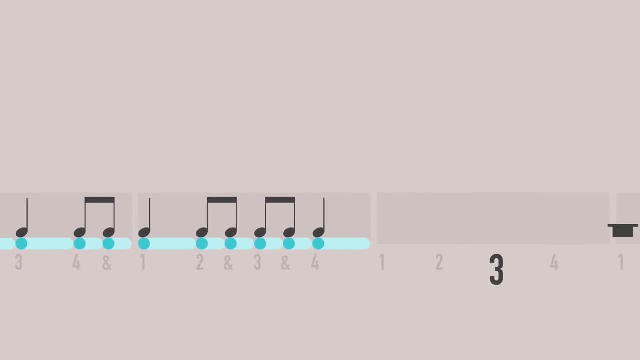 sound, then we can't just leave a measure blank. We have to use something called a rest. This is a whole rest and it plays silence over four beats. Rests work in exactly the same way as notes. A whole rest lasts for four beats. A half rest lasts for two beats. 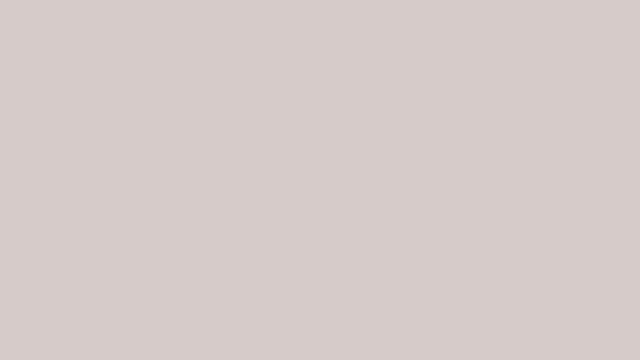 A quarter rest lasts for one beat And an eighth rest lasts for half a beat. Now that we have rests, let's play some more music. You might notice how it sounds different this time. Rests allow music. more breathing space. Again, we have to fill up. 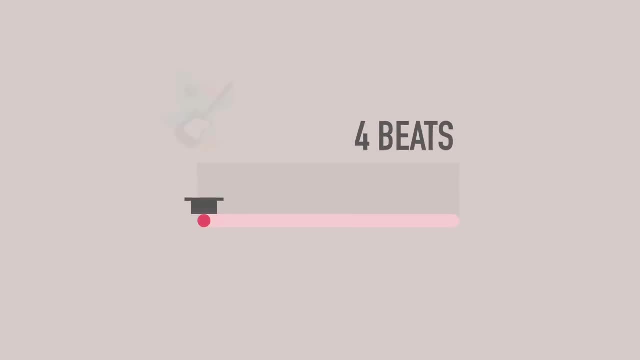 every bar with notes or rests and the beats have to add up to four. We can know that a half rest is enough to fill a body in a row. So a half rest is the number two bass, then the first fret or you.